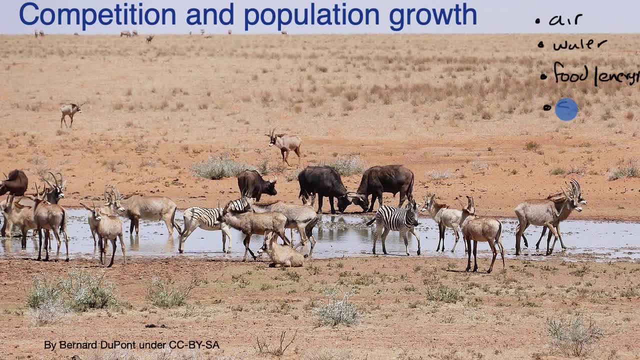 as we might recognize it, And I guess we think really, basically, they need space in which to exist. Now, as I mentioned, there seems to be a lot of space here for the animals, So that doesn't seem to be the resource that is limiting their growth. 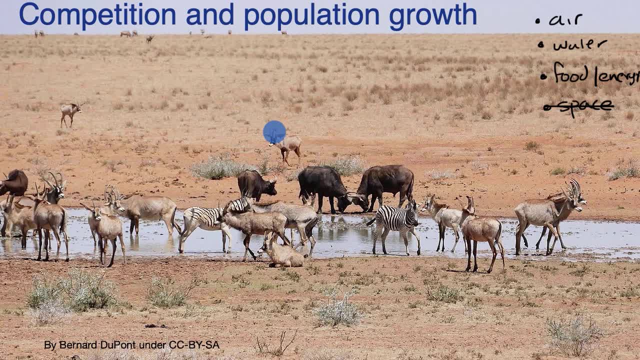 So let's rule that out here. Now it's also clear that it seems like there's a fairly large amount of air here, more than enough air for these populations to grow, So that doesn't seem to be a resource that's somehow putting a maximum. 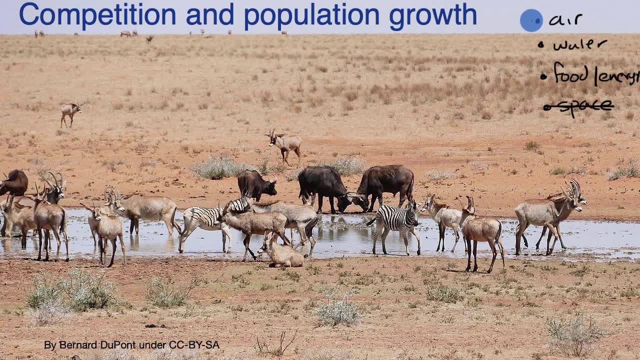 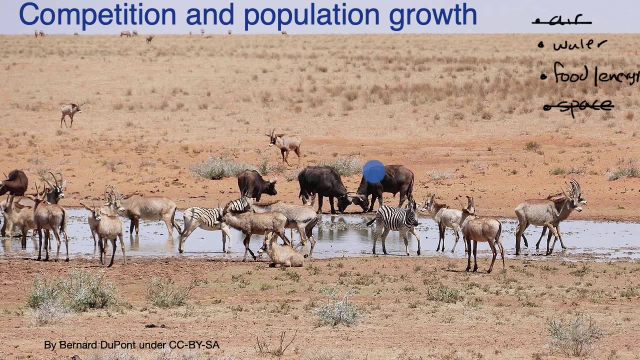 on how many of these organisms there are. It does not look like a limited resource or a limiting resource. Now, what about water? Well, water does seem interesting here, because this watering hole does not seem like it's very deep. It does not seem like there's a lot of water here. 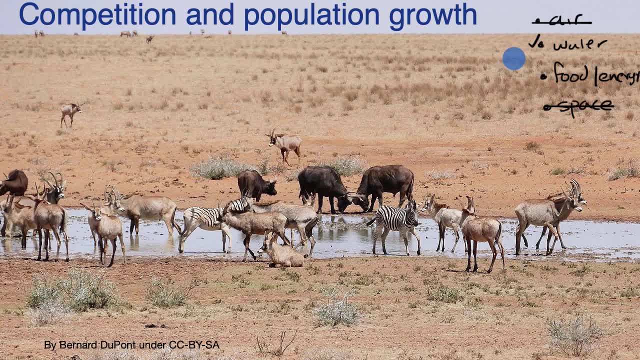 So this one could be what we would call a limited resource, that is, limiting population. Maybe if they had more and more offspring, there just wouldn't be enough water for any member of a population, And then, of course, the populations would be competing with each other as well. 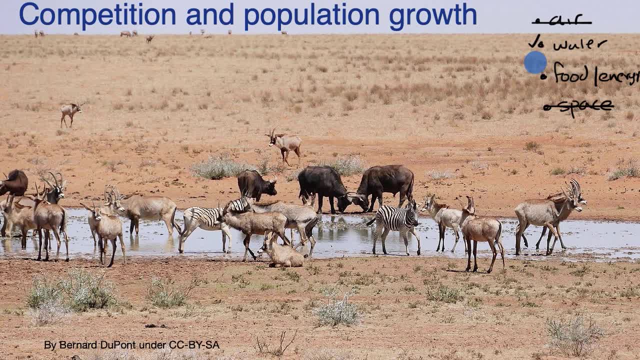 because they all need the same water to drink. Now, what about food? Well, you might recognize that zebra or antelope or buffalo. they tend to graze on grasses, And there are some grasses over here, but we also see that a lot of the grass is dead or dried out. 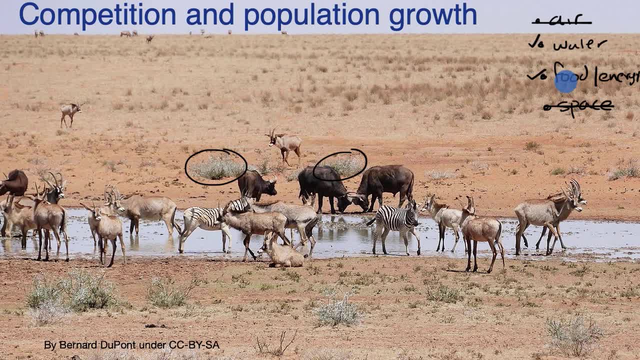 and there's just a lot of areas with dirt here. So it looks like the food and energy is also a limiting resource, And we have to remind ourselves. there's populations of different types of grasses, and why aren't they spreading more? 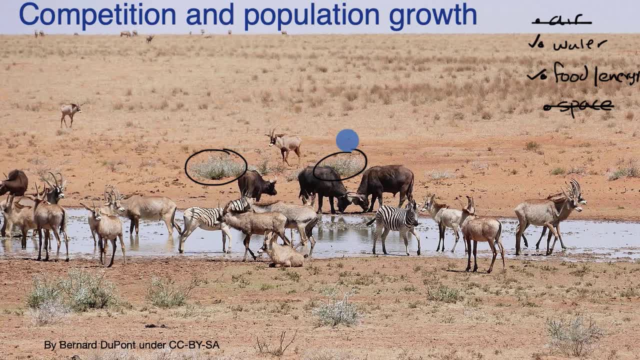 Well, from the perspective of a plant, it looks like the air and space is for sure abundant, and even energy in the form of sunlight is abundant, based on this picture. So it's probably water is the limited resource which is keeping us from having more plants. 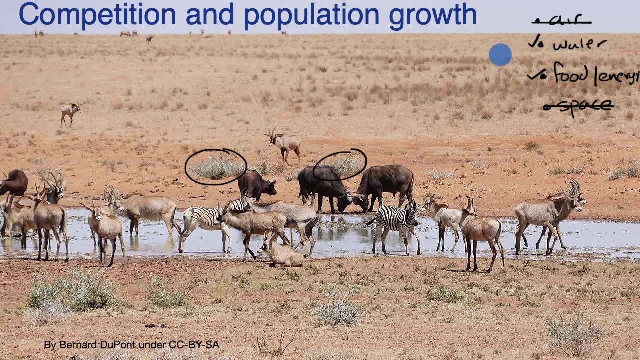 and grasses in this picture. We could imagine a scenario in which it rains a lot, there's a lot of water, water is abundant, then all of the different types of populations of grasses are able to expand and then there's more than enough food and water.